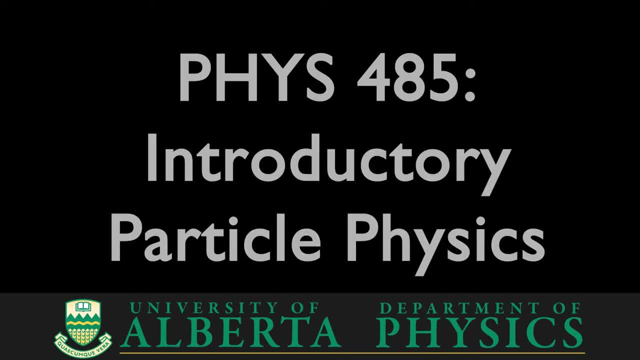 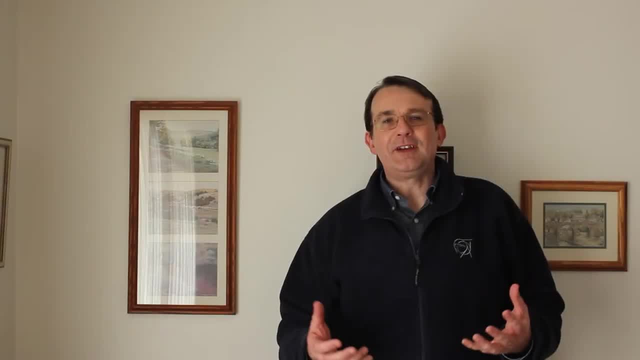 So in this video we're going to introduce the first symmetry of the standard model, which was discovered, actually, before we really thought of it as the standard model, And that symmetry is related to the flavor of light quarks or the flavor of nucleons inside a nucleus. Now 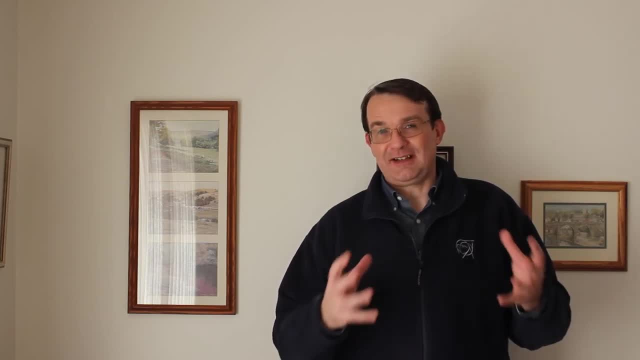 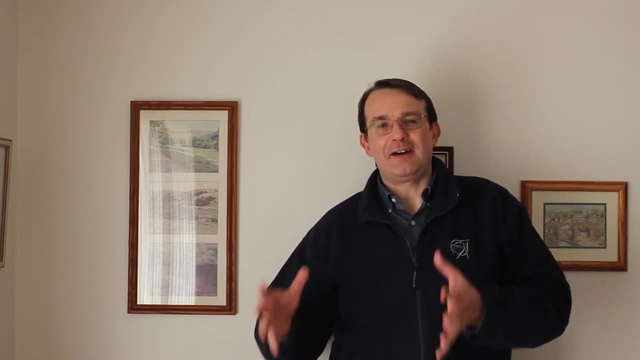 that symmetry is very similar, in fact identical, to the symmetry of spin half particles. So before we discuss our flavor symmetry, we're going to go back and refresh our memories about how quantized angular momentum works and how we can add two quantized angular momentum states to get a. 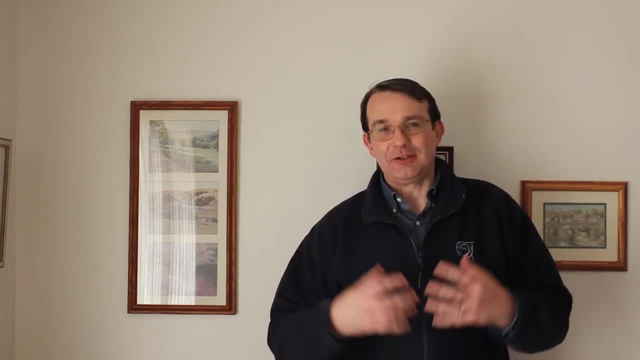 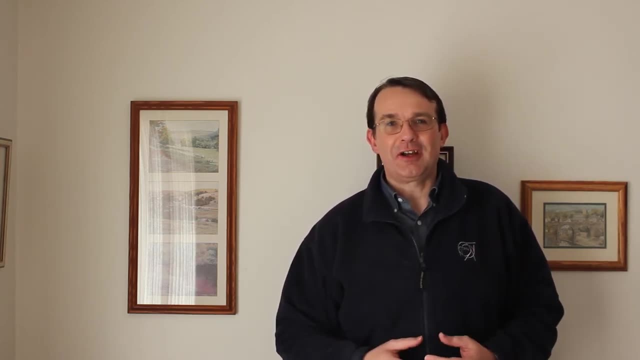 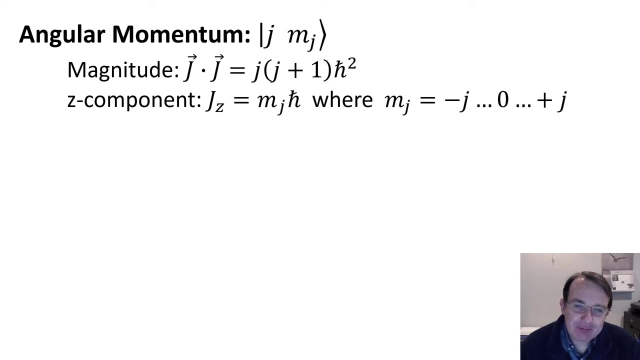 mixture of the total angular momentum state And that mixture of the states are connected through what we call the Klepsch-Gordon coefficients. So this is hopefully just going to be a quick reminder of quantized angular momentum. So when we're dealing with a quantized angular momentum, 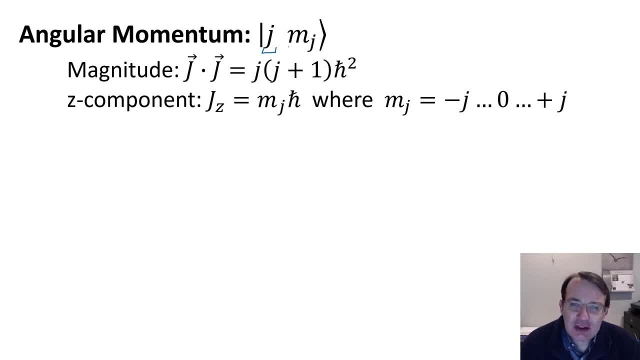 state. we have two quantum numbers, J and MJ. And J essentially gives us the magnitude And we can write down as the angular momentum vector, dotted with itself, which of course gives you the square of the magnitude, is J, J plus one times H, bar squared, So essentially the magnitude of our 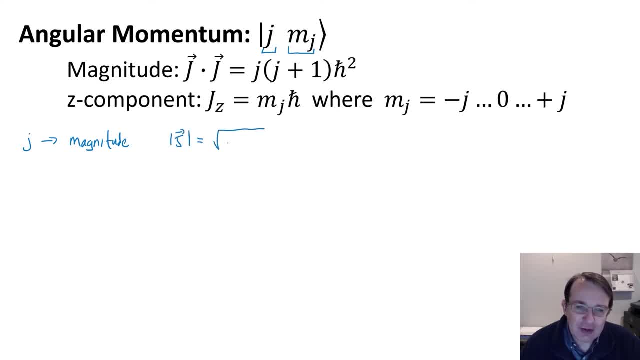 angular momentum vector is equal to the square root of J J plus one times H bar Right. And so we've got one quantum number that gives us the magnitude. Now the second quantum number, this M J here, gives us the Z component of the angular momentum. So J Z is equal to just MJ times H bar. 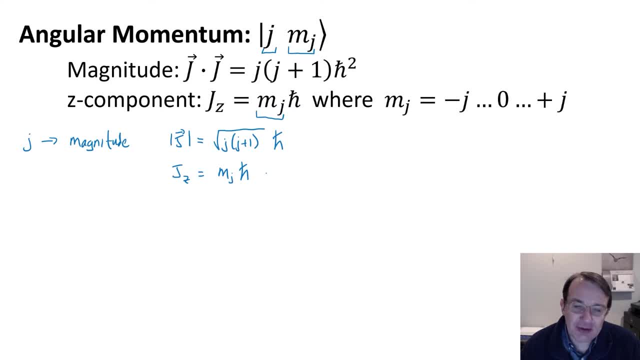 And so we have a single component of the angular momentum that's quantized. J X and J Y are not quantized. Only I mean we can obviously pick which direction Z happens to be in. I mean it's an arbitrary direction. But we only have one of the three components of our 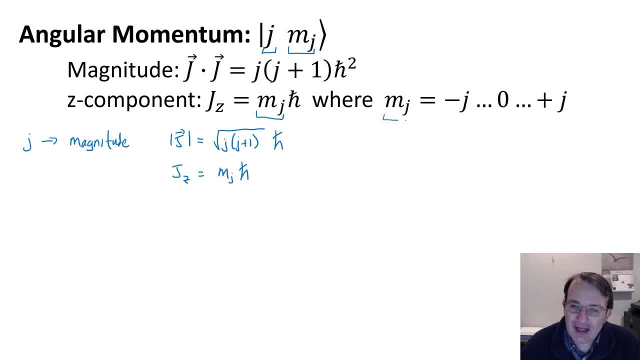 angular momentum which is quantized, And the rule on MJ is it can have any value between minus J up to plus J, any integer value. Now if your angular momentum has a half unit, it's possible, for example, to J to be equal to three over two. Then in that case MJ is minus three over two. 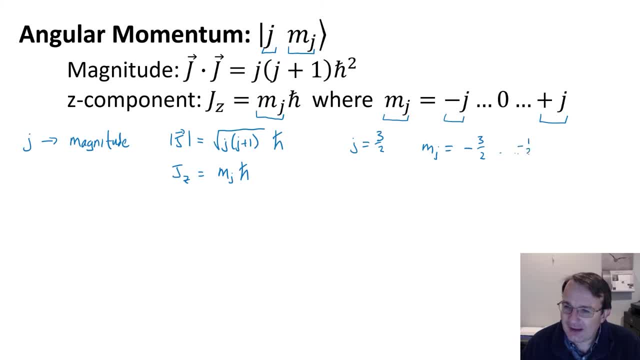 all the way up, but only going to minus a half And then plus a half and then plus three over two. So in this case MJ cannot be equal to zero. So if you have a half integer angular momentum, then your Z component cannot be zero, Right? 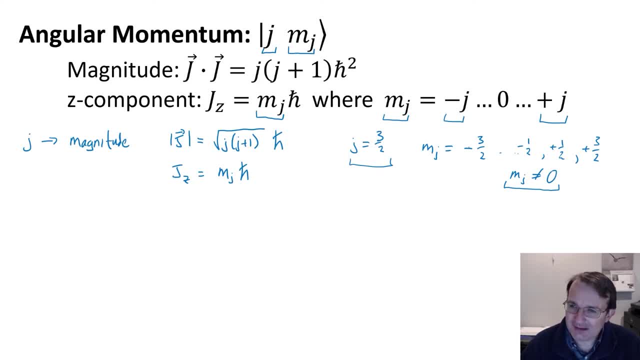 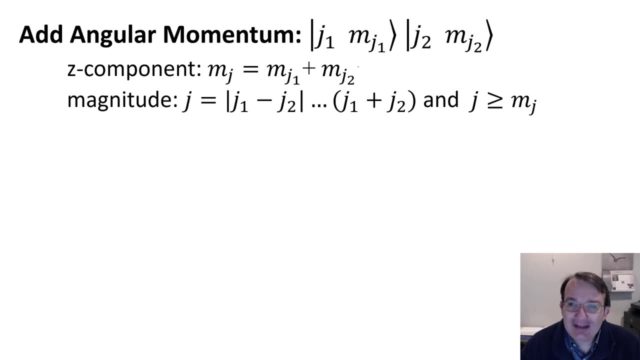 It also has to be a half integer and then going from minus J up to plus J, But obviously in this case zero is excluded. So that's a brief over reminder of angular momentum. And now we need to talk about adding angular momentum. So when we add two angular momentum, 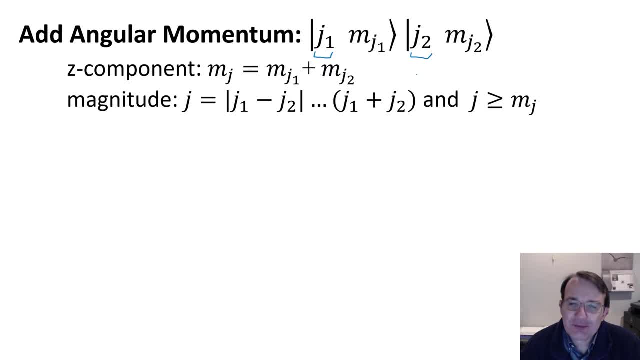 states. So here I've got a J one state and a J two state. Then the Z component of angular momentum is really easy because of course, obviously, when you're adding the two vectors, you just add the two Z components together, because those are the ones that we know. 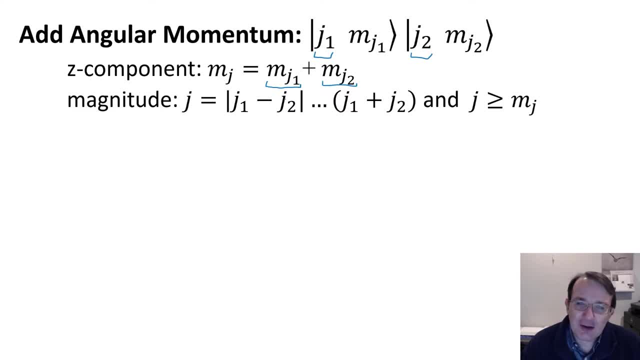 Those are the ones that are actually quantified and specified. So the final Z component is just the sum of the two initial z components. right, Just like adding an ordinary classical vector. The magnitude, though, is a bit more complicated, because the magnitude of the combined state 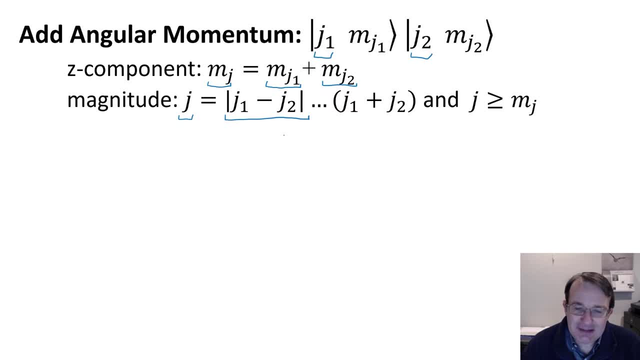 can be anywhere between the magnitude of the difference between the two, j1 and j2, all the way up to j1 plus j2.. But there is a requirement, of course, that j has to be greater than or equal to mj right. 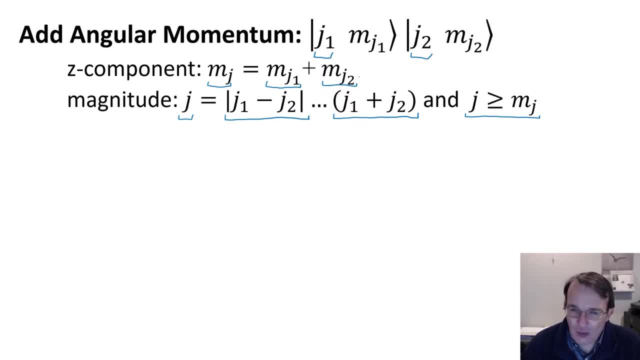 So, for example, if mj is 1 or mj is 2, then j has to be 2 or greater than 2.. It cannot be less than 2.. So those are the rules on adding them. So what this means is that when we add two of these states together, 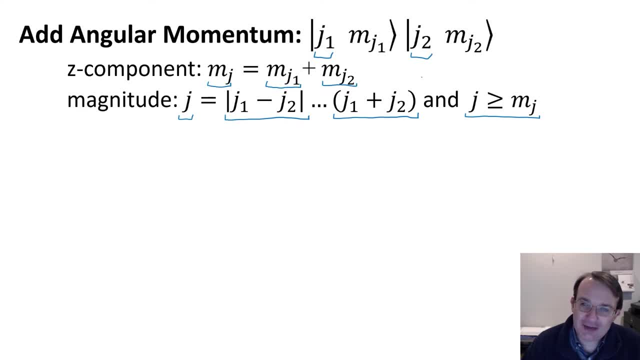 these two angular momentum states together and we want to know the angular momentum of the combined state. we don't get an unambiguous answer. We get a combination of possible states, all with the same value of mj here, but with potentially differing values for j. 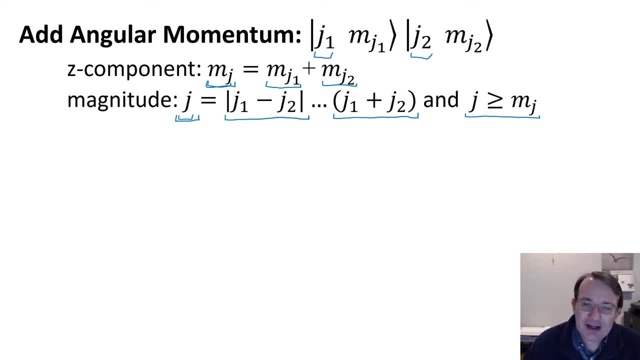 And the contribution of all the different possible states that go into this are determined by what are called the Klepsch-Gordon coefficients. So the Klepsch-Gordon coefficients are this thing here. So these are the Klepsch-Gordon coefficient. 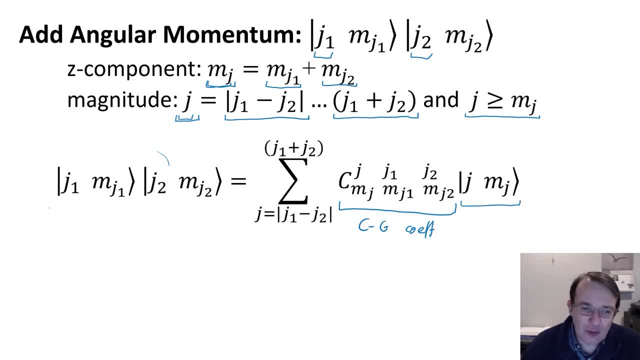 And then this is the particular state. So when we combine these two angular momentum states, we end up with a sum over here of these Klepsch-Gordon coefficients times each of the allowed combined states, And so the contribution from each of these different states is determined by the state. 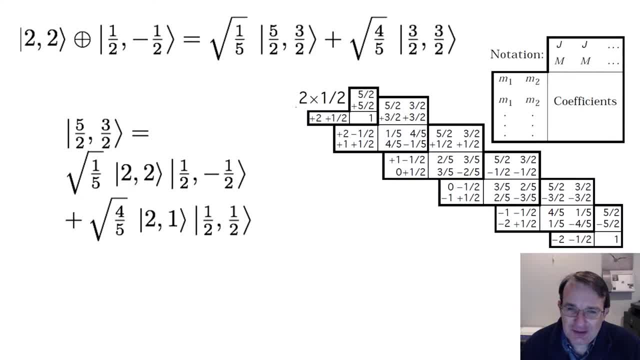 And so the total state is defined by these coefficients. Now, to determine the Klepsch-Gordon coefficients. we do not calculate them. We have these handy tables that are provided by a particle data group, And so these are the tables we're going to use. 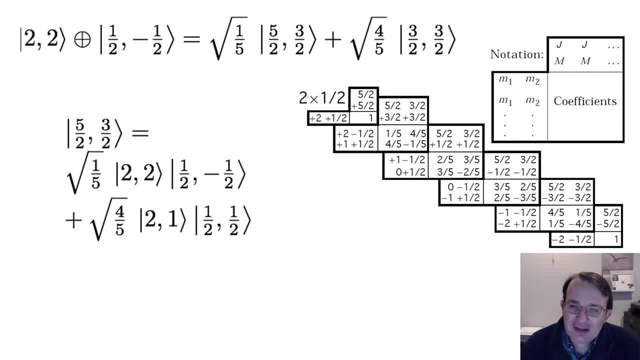 when we have to deal with the Klepsch-Gordon coefficients. So each table that you see- and here is one of such table shown here, so this is the table- Each of these tables is a combination of two different angular momenta. so, or as we'll see, something else, so this is, for example, J. 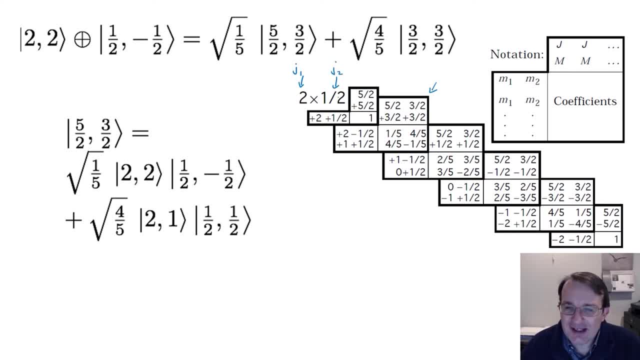 one, and this is, for example, J two. so this is the table you use when you're combining a spin two particle with a spin a half particle. right now, the way this works is there's two ways you can use it. so what you can do is you can say: 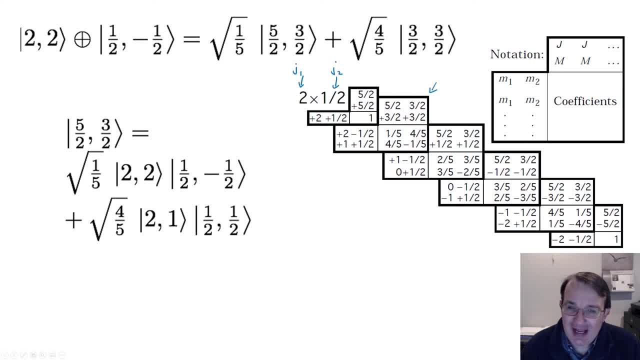 well, I know the initial states of the two particles that I'm adding together, right? so obviously you have to know j 1 and j 2, but then if you know the initial states, then you also know MJ 1 & MJ 2, and so these are the M numbers here. so this, for example, will be M 1 and this 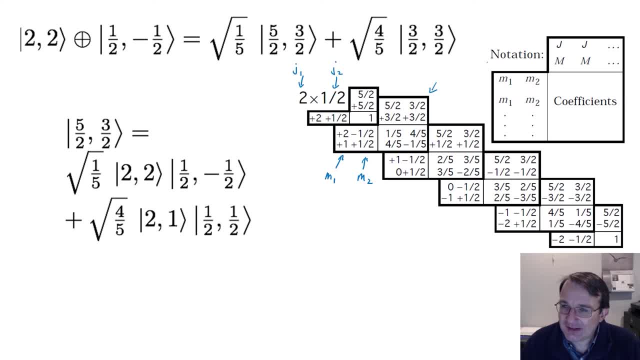 column here is n 2, as you can see here. you know, in the notation list these are the M numbers on this column here. those are the m1 & m2 numbers. so in the notation list these are the m numbers here. so these are the m numbers here. so these are the m numbers here. 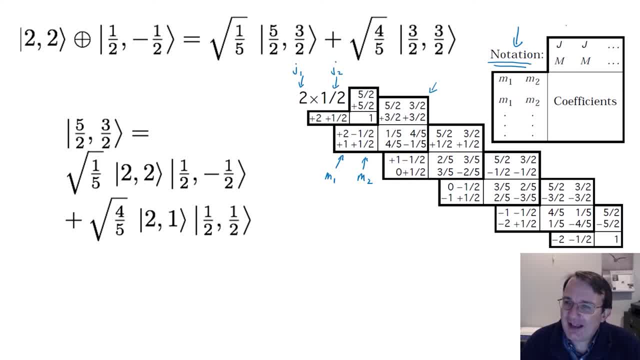 numbers go down the side for the initial states and then the other column. here is the total momentum of the combined state and the total z component of the combined state. So what this is telling us, so if we look here is we, if we start with a spin, 2, so this is remember, j1 and this is. 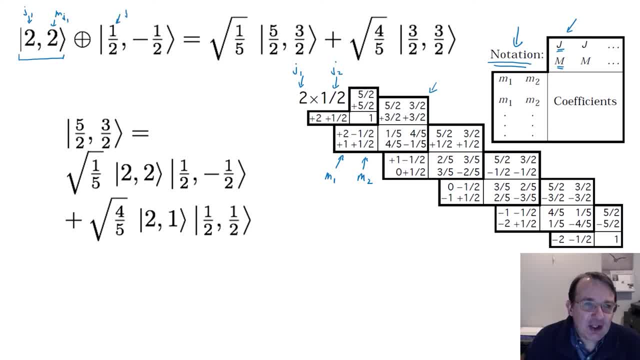 m j1 and this is j2 and this is m j2.. So we've got the two and the half. well, that's why we're using this. two cross a half table and then we have: m j1 is two and m j2 is minus a half. So we look. 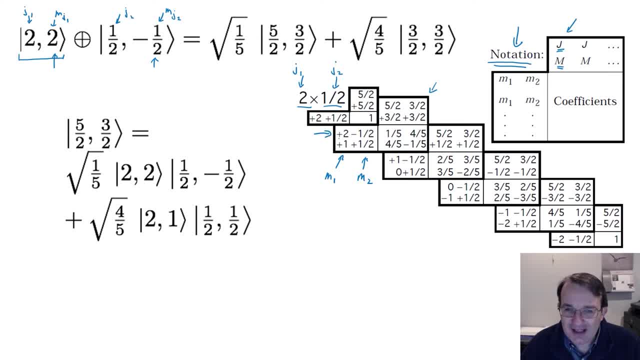 at this row here, because that has m j1 equal to plus two, which is what we've got, and it has m j2 equal to minus a half, which is what we have. And then we see that along this row, we then see these two coefficients, one over five and four over five. Now the way the particle data group have written. 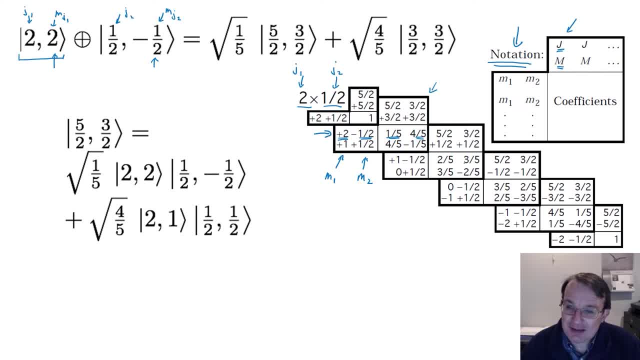 these is that for any one of these components there is an implicit square root. So if I take, for example, this minus four fifths here, the way that is interpreted is as minus the square root of three. So if I take, for example, this minus four fifths here, the way that is interpreted is as minus the square root of. 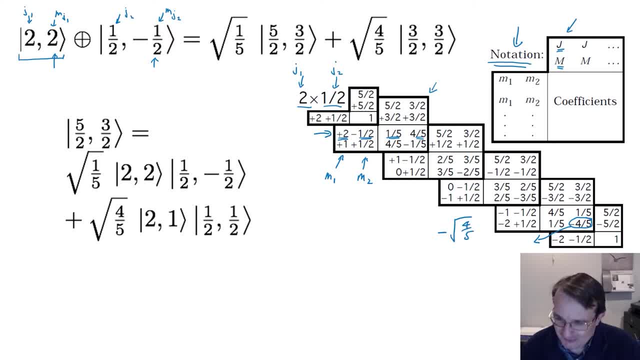 four over five, not the square root of minus four over five. right, the minus goes in front of the square root and then you put the square root around the term. so two-fifths here is actually the square root of two-fifths. minus a half is minus one over root two. um, oh, sorry, that's actually. 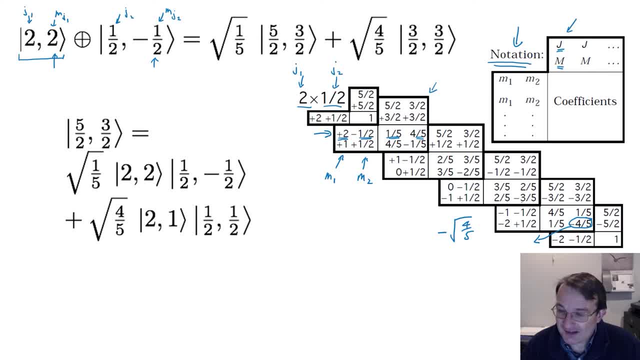 one of the coefficients. so minus three-fifths is minus the square root of three over five, right, um. and so that's um how we interpret these coefficients. and so if we look here we can say: well, this minus a fifth belongs to the state where j is five over two and mj is three over two. so 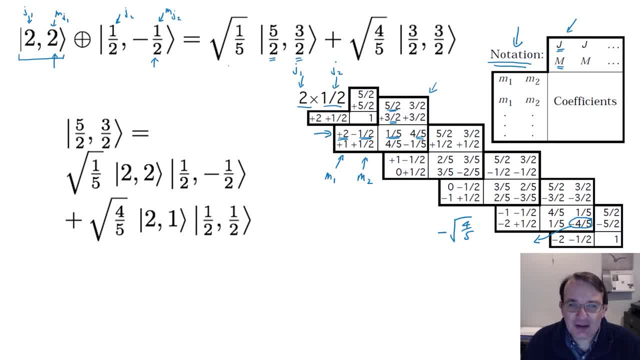 five over two, three over two and that has a coefficient of square root of one over five. and then we have this other contribution which is square root of four over five. so that's the cleps gordon coefficient here. and then this is of the state three over two. uh, j equals three over two and mj equals three over. 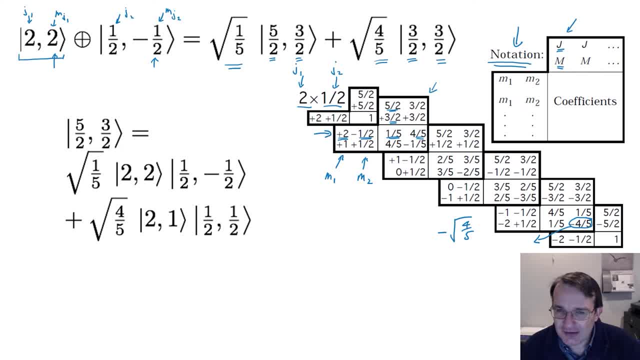 two, and so we can see j three over two, mj three over two. so that's how we can use the table um, when we're combining two known states and we get the mixture of two, you know we don't get a single uh total angular momentum state, we get a mixture, mainly this angular momentum state, but a. 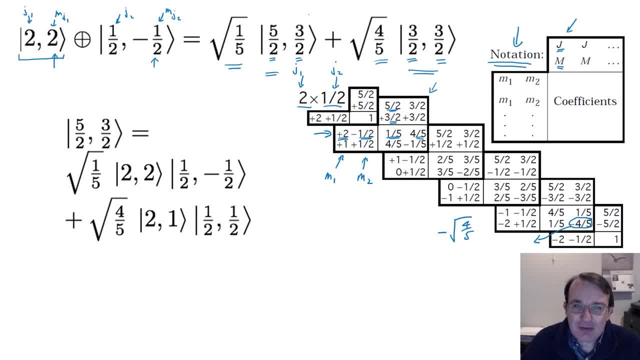 little bit of this angular momentum state and, as you can see, here we've got a mixture of the two, so we can see both of these states have the same value for mj, because mj has to be equal to two minus a half. right, it's the j value that this differs. we have a five over two and a three over 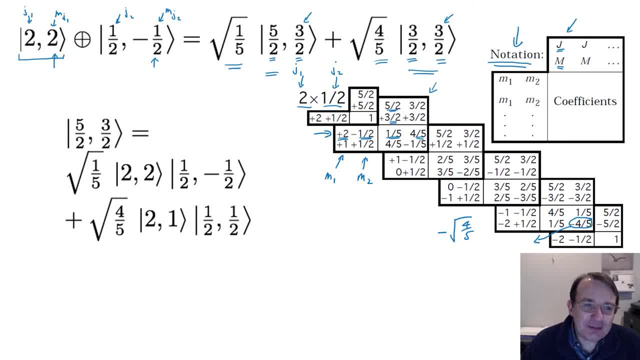 two. now we can also do that in reverse. we can say: well, supposing i have an initial state where i know the uh, the j value and i know the mj value and this, you know, maybe it's a particle in this state that decays into two particles: uh, one with spin, two and and. 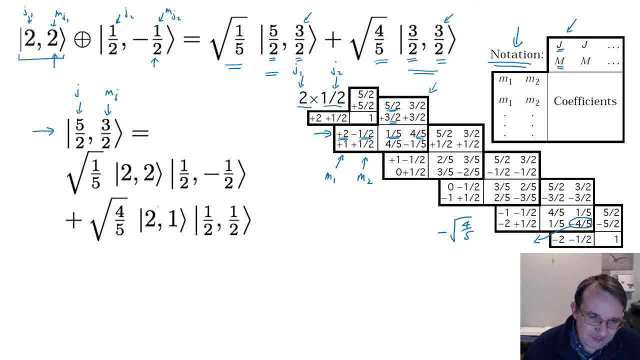 and uh, mj two and one with spin a half, um and mj- well, the sorry one with spin two and one with spin a half. and then we don't know what the ratio of the mj values are going to be for each of these particles. so now i'm going to start looking on this side, and so i want the column. 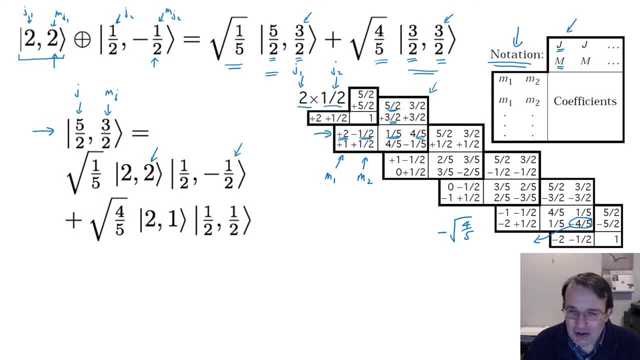 now that has j equals five over two and mj equals three over two. so that would be this column here. i've got five over two here and i've got uh three over two for for mj, and so this tells me that i have a coefficient of uh one over the root, uh one over root, five for uh, you know, m1. 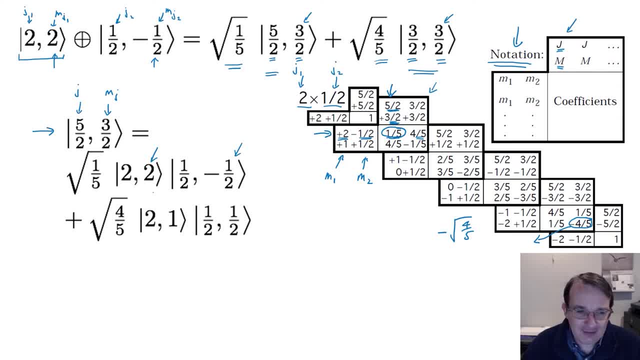 equals to to plus two and m2 equals plus a half, right, so m one or mj one is equal to plus two, mj two is equal to minus a half, and i have one over root five for the coefficient, just like i have here. then i have this coefficient here, so square root of four over five, and that 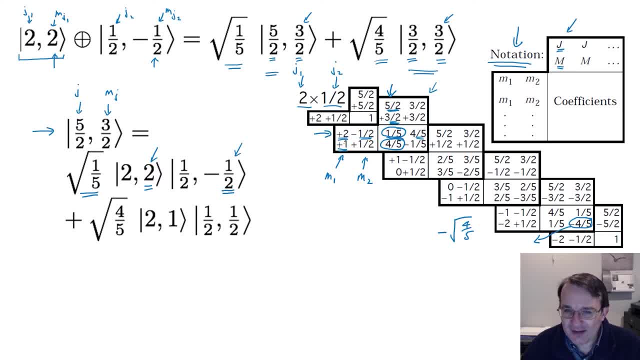 is for a state where, um, m uh one is plus one and mj two is plus a half. so mj uh one is plus one, mj uh two is plus a half and of course the other spins of the two particles are, and of course the other spins of the two particles are. 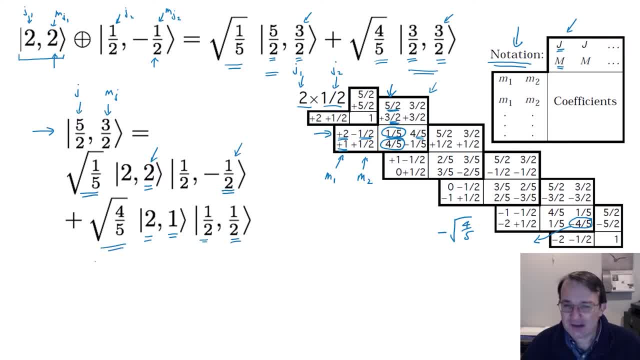 determined, and this is the coefficient square root of four over five. so you can use these tables to either split a combined angular momentum state into its uh, into its two components, or to combine two components into a single total angular momentum state. so you can use these tables either way, just make sure that you pick the. 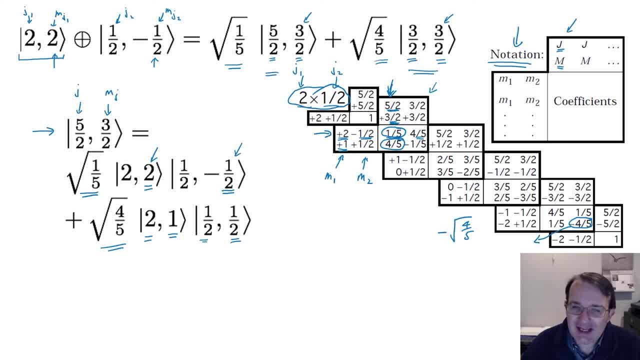 right table for how you're splitting things up. so this is again splitting things up into a particle with spin two and a particle with spin a half being either split or added together, depending on which way you're using the table. now this is just a a brief discussion of a special 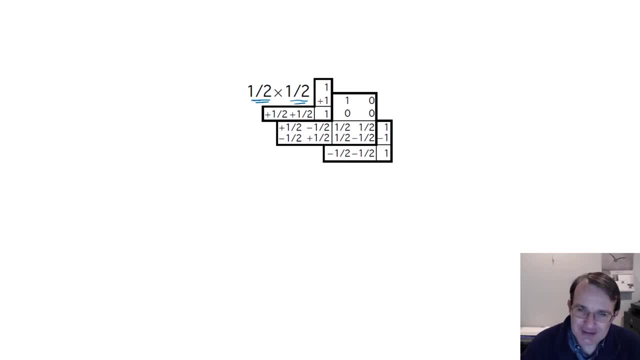 case, and that's where you have two spin a half particles being combined. now, in this case, you only have four different outcomes, right? because you've only got two spin a half particles and each of these spin a half particles can only have, you know, mj equal to plus or minus. 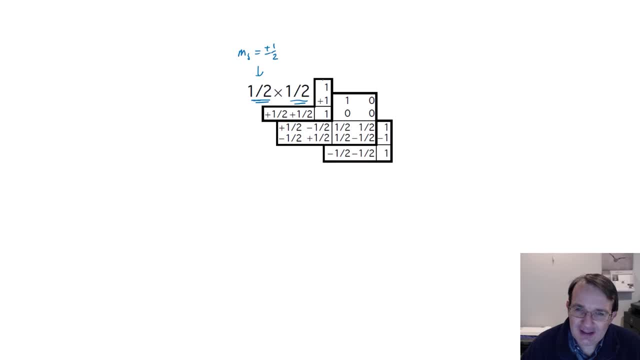 a half, so there's only four possible uh outcomes, and what's interesting to note here is that you have what's called the triplet state, right, and the triplet state is where there are three possible states, all with the combined momentum equal to one, and then you have a singlet state here where 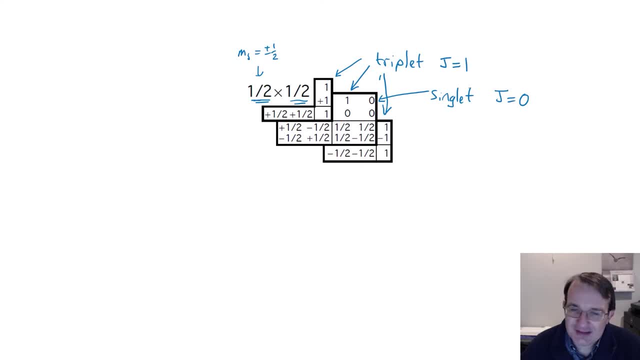 the combined momentum is equal, is equal to zero, and so this is a pattern that is often seen, where you can combine uh, two particles, you end up with three possible j equals one states and only a singlet j equals zero state. but you get similar sort of splittings and numbers of states depending on the angular momentum of the particles. 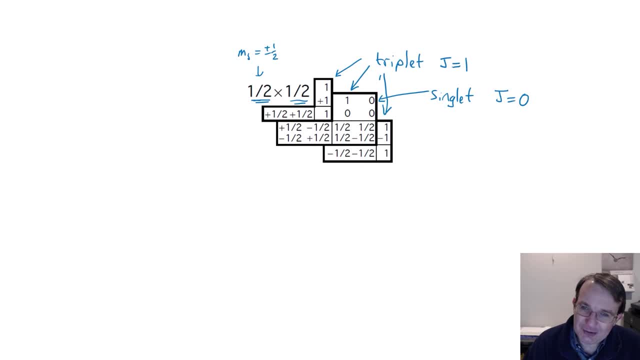 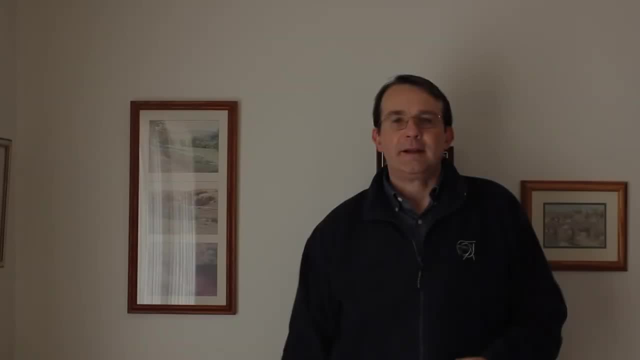 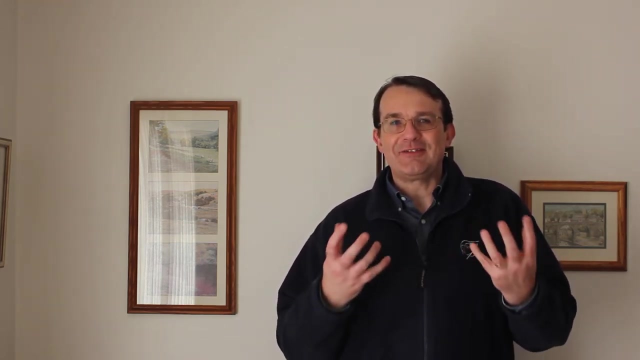 that you're adding. so this is a special case. for spin two. you get a triplet state with j equals one and a singlet state with j equals zero. now we've seen how to combine two separate quantized angular momentum states to find the mixture of total angular momentum states. that's equivalent to the. 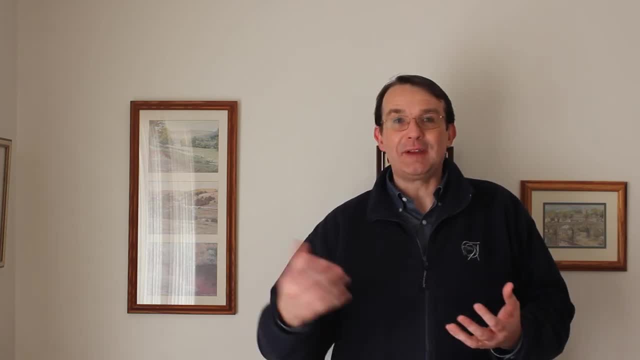 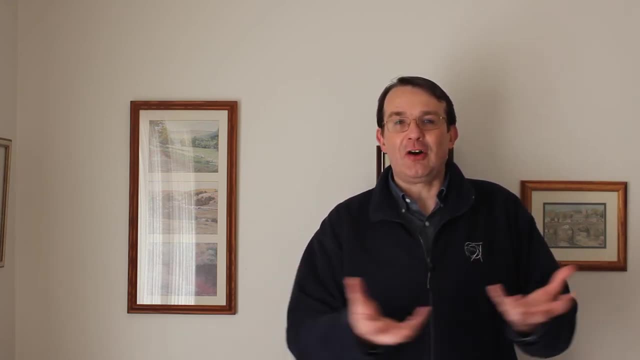 two separate states. and we've also seen how we can do that in reverse. if we start with the two angular, the total angular momentum state, we can split it into the mixture of separate states that combine to give that. and that is all through these cleps. gordon coefficients: now, if we're dealing with spinner half particles, 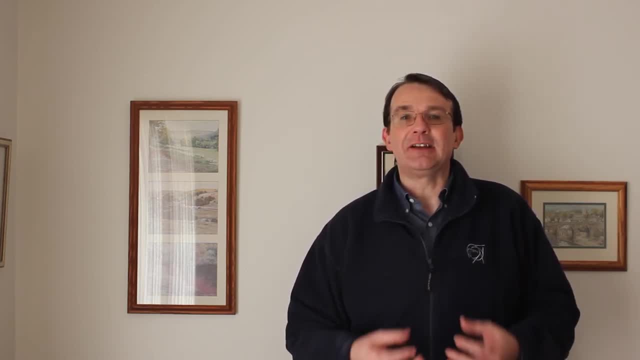 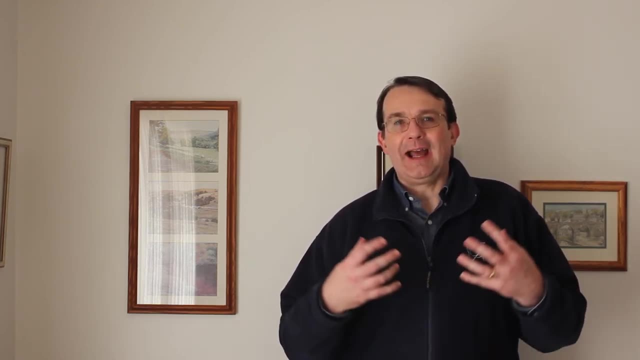 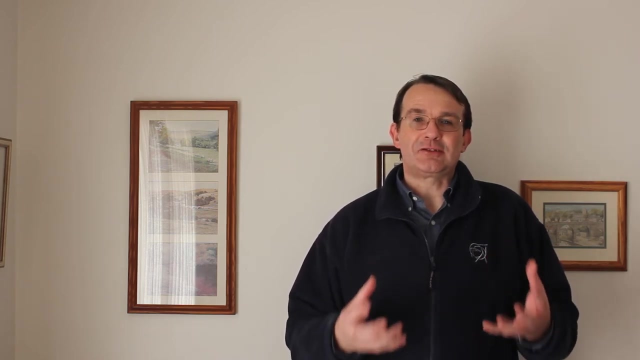 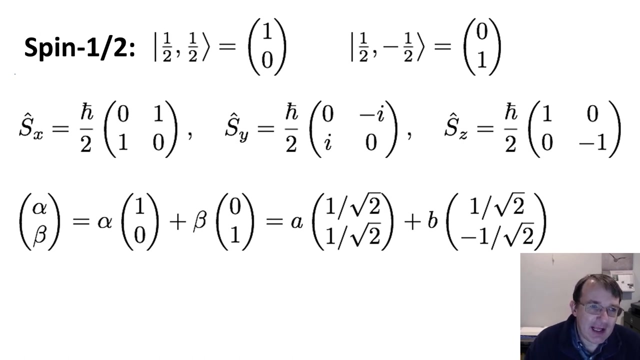 we can actually represent the spin state of the particle as a two component vector that is called a spinner, and that spinner can be operated on by spin operators to extract the x, y and z components of the spin. so let's see how that works now. we can represent the spin states by the uh a vector called the spinner, and 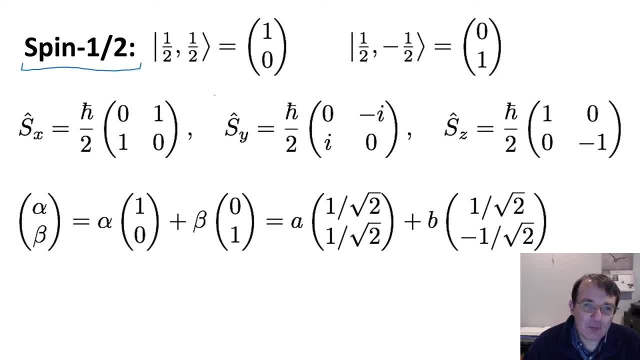 when we're dealing with spin a half particles, we only have two possible states, um, and so that's, for example, remember, this is uh, j and this is mj, and so we have j, equals a half, and then we have mji, equal to half minus a half, and so we can represent these spin a half states as a what's called a spinner vector. 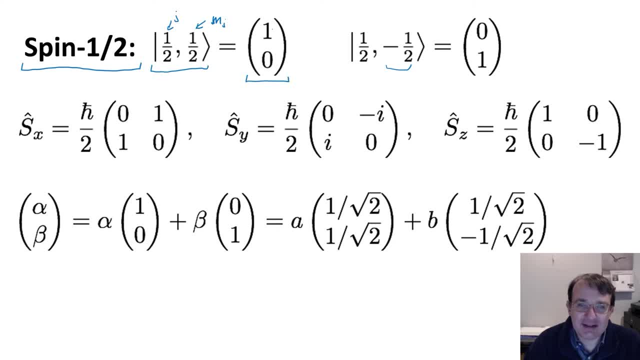 and we can represent the spin up state as 1: 0 and the spin down state as 0: 1. and remember- this only applies when we're dealing with spin, a half particles- that we can represent it as this sort of two component vector. now, if we do that, we end up with three spin operators, and so this is the x. 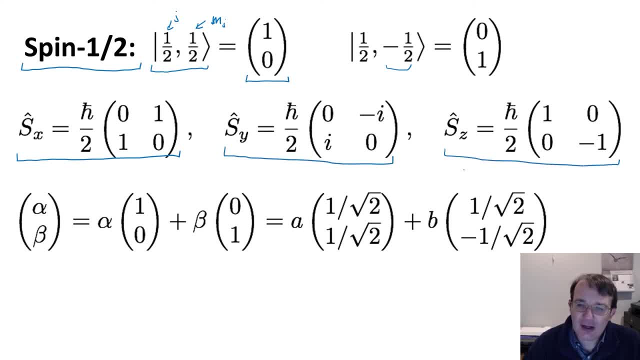 the y and the z component of the spin operators. and it's easy to see that if we're using sz here on these states where, remember, this is the z component that's quantized, then we end up with operating sz on these two states, spin states. we end up with quantum numbers for the z component of the spin of equal to plus or 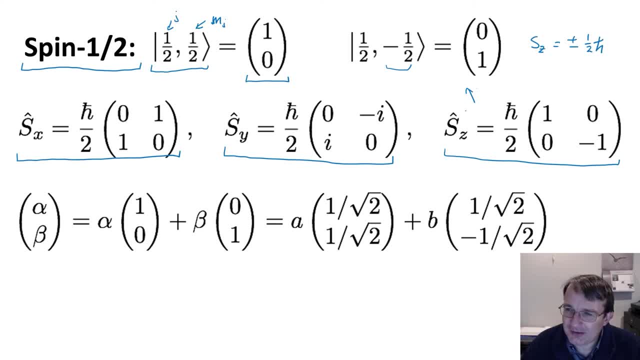 minus a half h bar or h bar over 2, so we end up with these. so these are the eigenvectors of the z component of the spin and these, essentially, are their eigenvalues. now, if we do that for the x or the y components, or if we do this, for example, 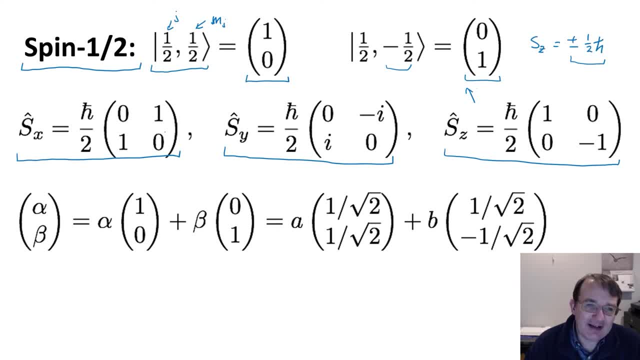 let's start with the, let's concentrate on the x component, then the eigenvalues, or the eigenvectors. for x, the quantum numbers are the same. we're still going to get s, x as plus or minus a half h bar, but the eigenvectors are different. right, and so we get in fact, for, for sz, we get one. that's essentially 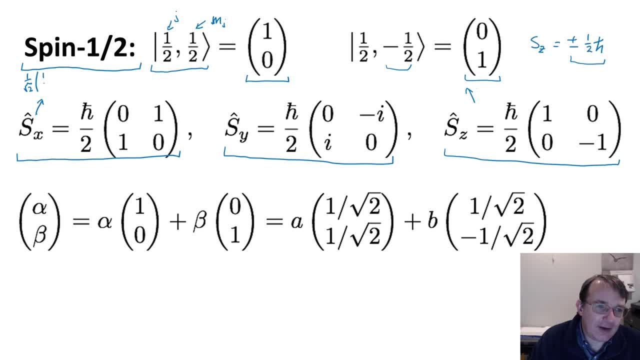 one over root, two of one, one, and then we get one that's essentially one over root, two of one one, and the other one is one over root, two of one minus one. so the uh s, x, uh operator has different eigenvectors but the same eigenvalues, and we can write a general spin state. so if we've got our 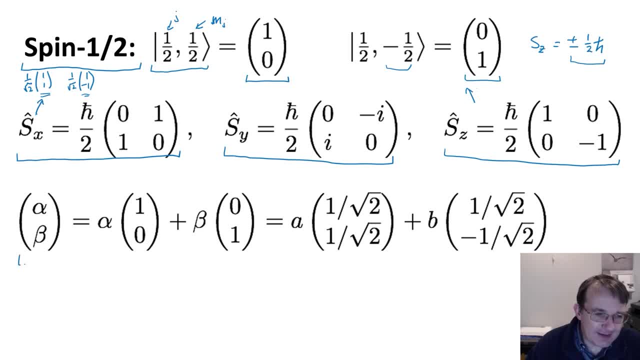 spin a half particle in an unknown spin state. we can write this as alpha, beta, as the two components, and so then it just becomes, you know, alpha times uh, one, zero, and beta times 0,, 1, but we can also express that in terms of the eigenvectors, for example of the 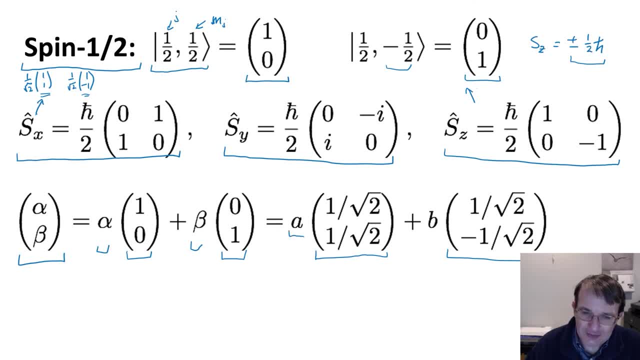 x spin operator. only then, of course, we're going to get different coefficients, a and b, and we know, since it has to have whatever this state is, it has to have, it has to be, you know, either in this state or in this state, if we're looking at the z component, so that tells us that. 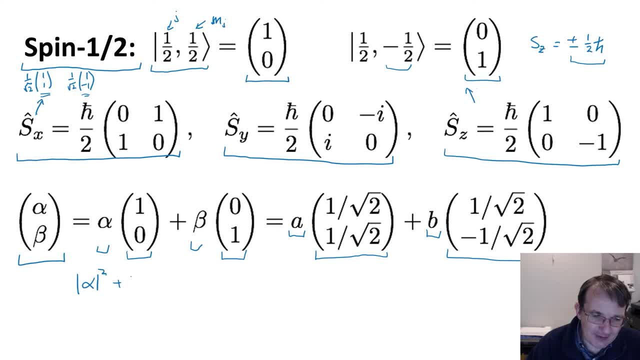 the modulus of alpha squared plus the modulus of beta squared has to be equal to 1, because the modulus squared here gives us the probability that it's in this state versus the probability that it's in this state and it has to be in one of those two states. So this is sort of our 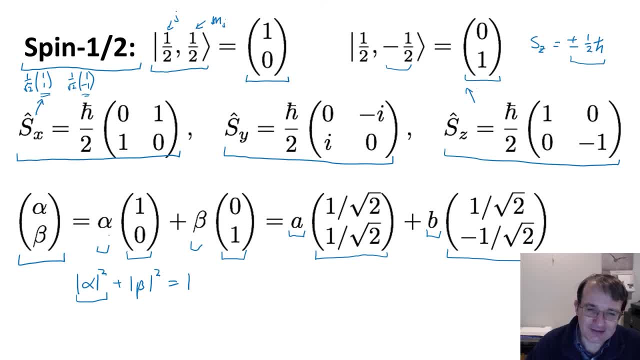 unitary condition, but we can use these components to find out the probability. Similarly, we can do the same for these a and b components. So what we're going to do is we're going to do the same thing with the sx state, and so what you can see. 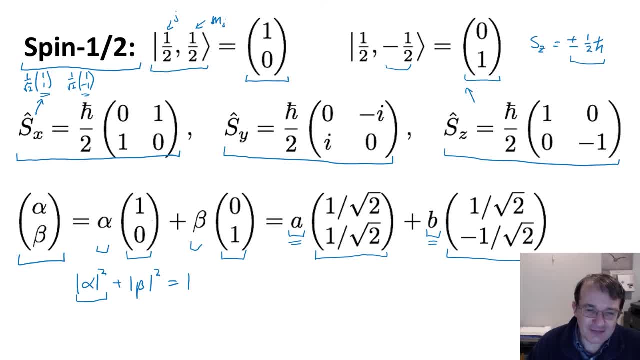 here is that if, for example, I'm in an eigenstate of the z component of spin, when I express that so, here beta would be 0, when I express that in terms of this, here I'm going to actually have equal mixtures of these two right in order for the y component, you know, the bottom component. 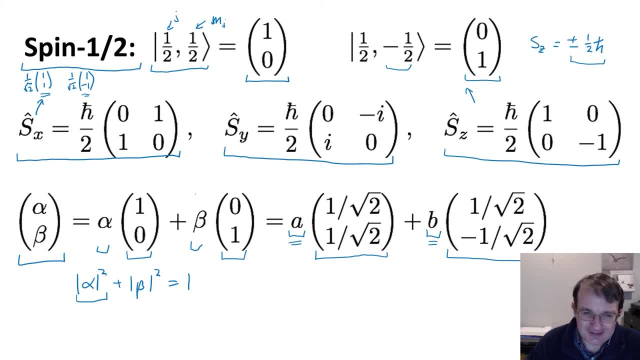 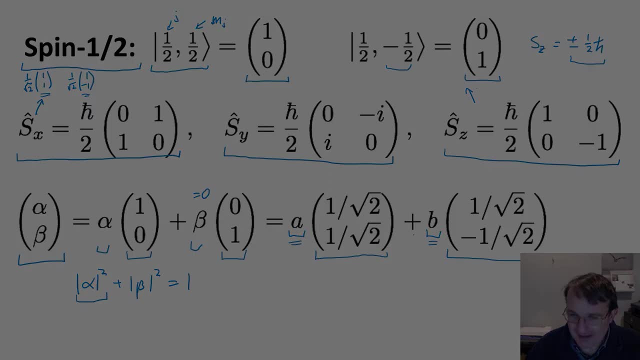 of the spinner to cancel out, to give me 0 here, That's in the case where beta is equal to 0. I need these two to cancel out, so a and b will be equal, and so that tells me that you know, if I've, if I know, my z spin, then I've literally no idea. 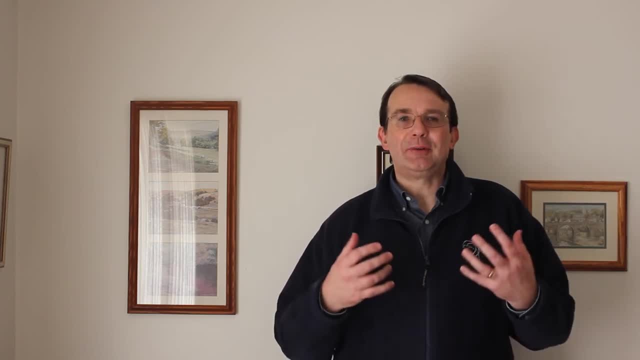 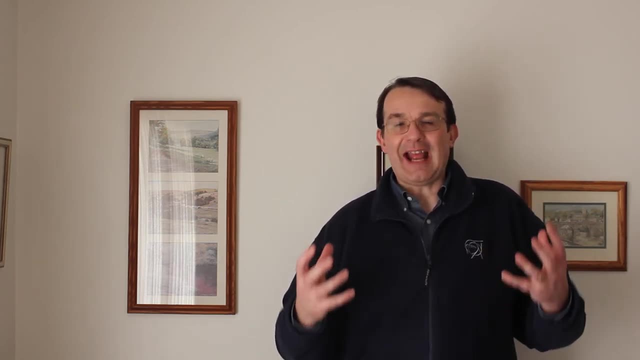 So now we have all the tools we need to examine the first flavor symmetry of what became the standard model. Now, this is actually a fluke. It's not a fundamental symmetry of nature, it's more an accidental symmetry of nature. So what we're going to do is we're going to do a little bit of a symmetry that comes about because the mass of the neutron and the mass of the proton just happen to be almost identical. They're not precisely, so. it's not a perfect symmetry, but they are very, very close to one another, and that equivalent in mass means that we can pretend that there is a single. 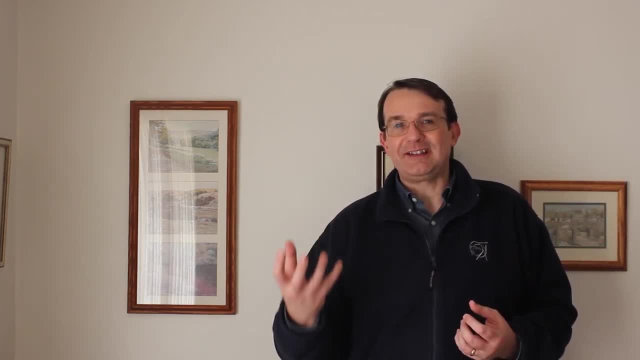 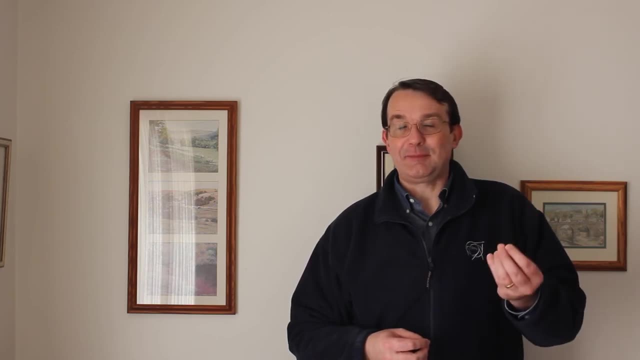 nucleon particle and we can think of it as existing in two states, a neutron and a proton. In just the same way, we can have our spin a half electron exist in two states: spin up and spin down, And, in fact, 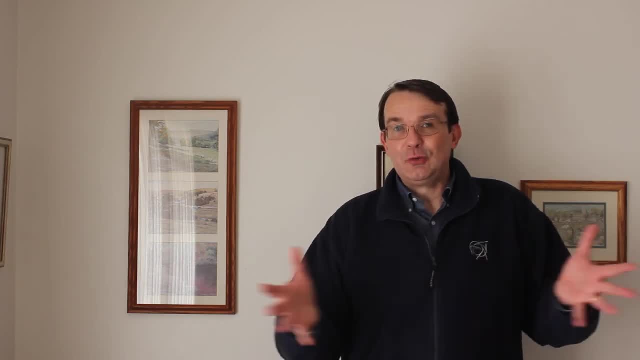 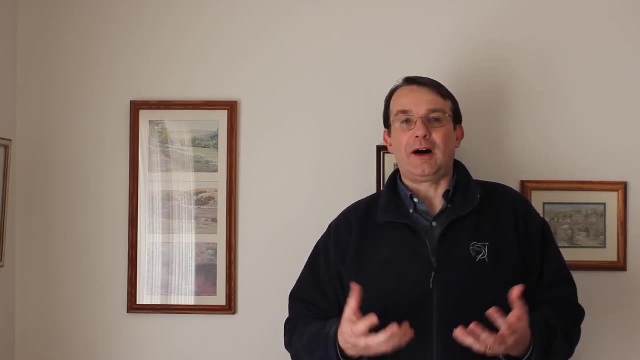 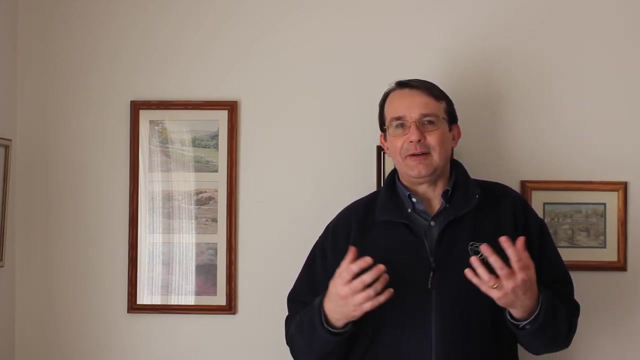 at a fundamental level, we think of this as the two lightest quarks, the up and the down, as having basically the same mass, And so we can think of this as a single light quark that exists in two states, an up state, which is the up quark, and a down state. Now, it's important to remember that. this is a fiction, right? It is not. we don't actually believe that there's a single particle with two different flavor states. We think of them as two separate quarks, But because the masses are so similar, we end up with a symmetry that works if we pretend that there is a single particle. a light quark that can exist in one of these two states And in fact that's where the names up and down probably came from. is that we have it in an up flavor state or a down flavor state? And the name of the symmetry because of its similarity to angular momentum and spin. 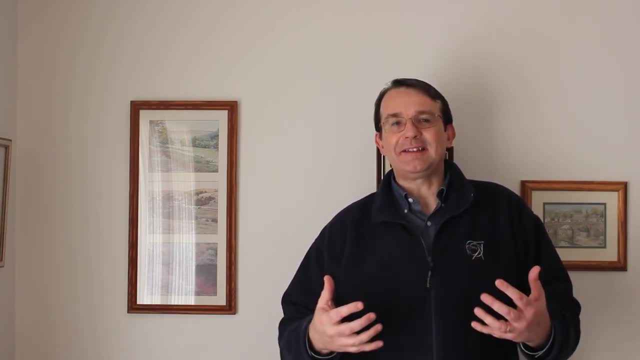 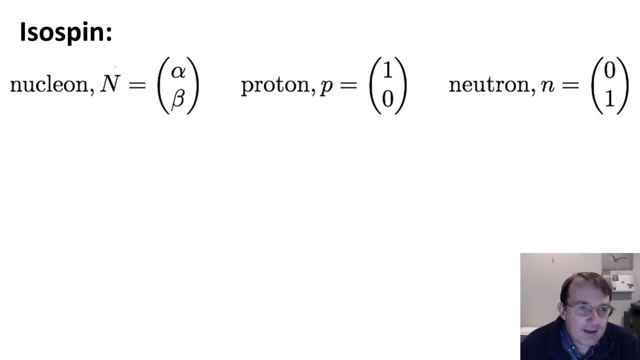 is called isospin. So let's see how we can construct isospin for the nucleons and the quarks. So now we've talked about spin a half particles, we can introduce this thing called isospin, And this is nothing to do with angular momentum at all. It has literally nothing to do with angular 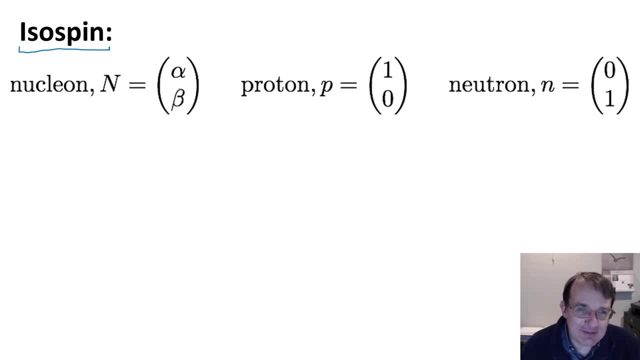 momentum, But, as we're going to see, it has the same symmetry and the same rules as angular momentum, And that's why we think of it. we call it, in fact, isospin, even though it's actually got nothing to do with angular momentum at all. It's entirely an artificial construct used to describe flavor. 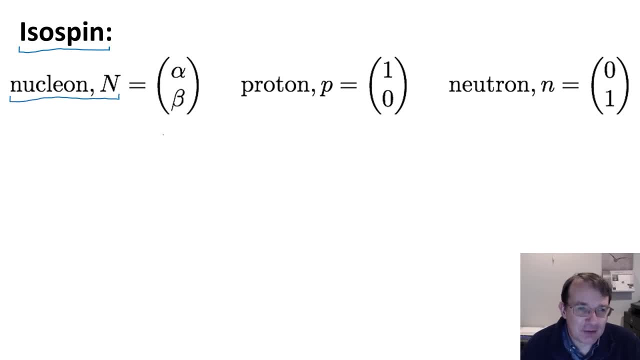 And so what we imagine is that there is a particle called a nucleon- And this are the particles that we find in atomic nuclei- And this nucleon can have a isospin, an isospinner alpha, beta here, And the nucleon can exist in one of two. 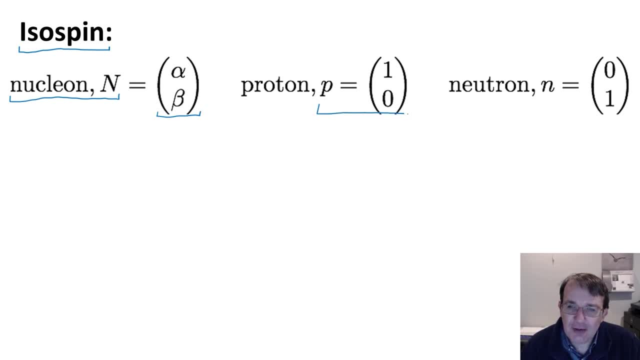 states: Either the nucleon can be a proton, in which case its isospin vector is 1, 0. Or this same imaginary nucleon particle can be a neutron, in which case its isospin vector is 0, 1.. 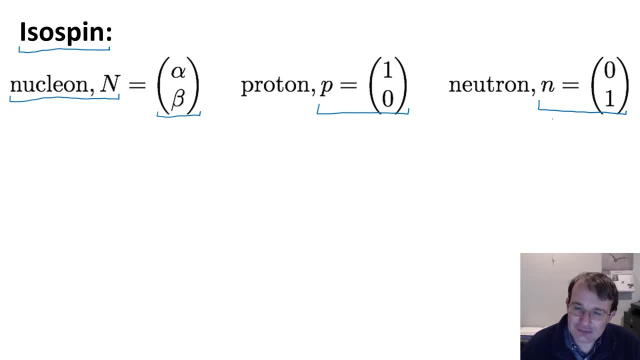 So what we're doing here is we're thinking, if you think of it, like an electron can have spin up and spin down, right, And that's a physical angular momentum state. What we're saying here is we've got a nucleon and it can exist as a proton or a neutron. So again, 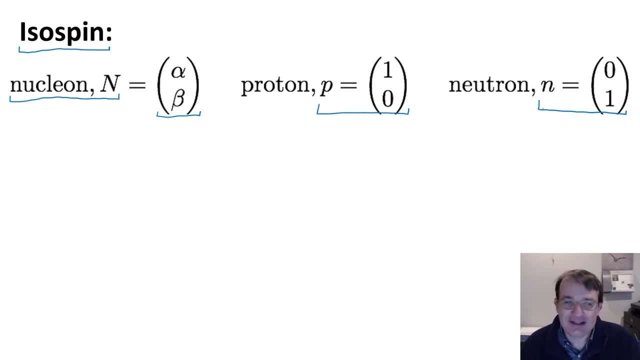 just like the electron can exist in two spin states, the nucleon can exist in two flavor states, either a proton or a neutron. And if we write these out in terms of the isospin states, then we're going to have a isospin vector, And so what we're going to do is we're going to 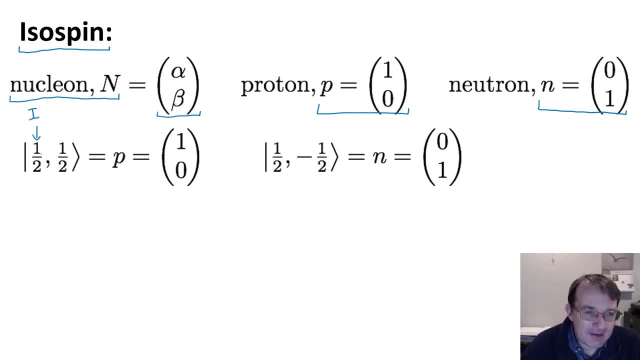 this number here is the magnitude of the isospin. So for a proton we have isospin a half, And this is the third component of isospin. We don't call it the Z component because isospin is not a real vector, It's not like an angular, it's not angular momentum at all. 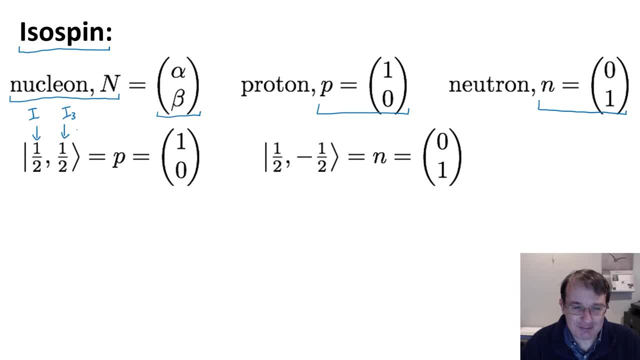 literally no association with angular momentum. But the mathematical patterns for angular quantized angular momentum match exactly the same patterns as we have for isospin, at least when we have spin a half particles. So our proton here has isospin magnitude a half. 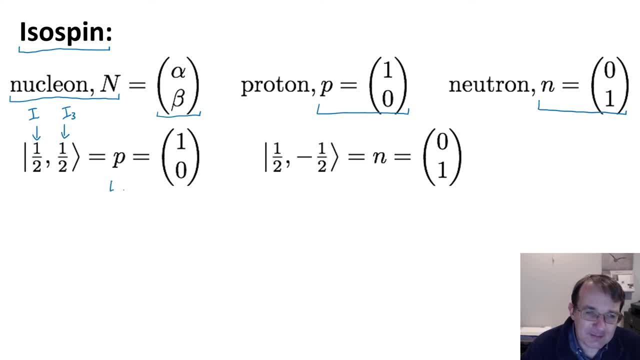 and I3 equal to a half, And this gives us a proton with its isospin vector. For the neutron we have isospin, again a half. But now the third component of isospin is minus a half, And then that gives us a neutron with its isospin vector. 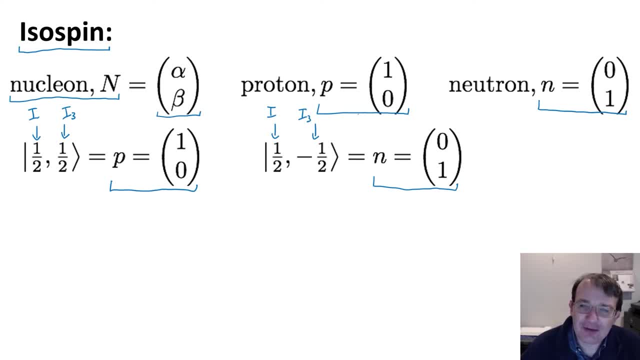 So now you know this accident comes about and this is how isospin started- because the proton and the neutron have almost identical masses- not exactly identical masses, but close enough that we can think of them, or we can imagine them, to be a single particle in two possible states. 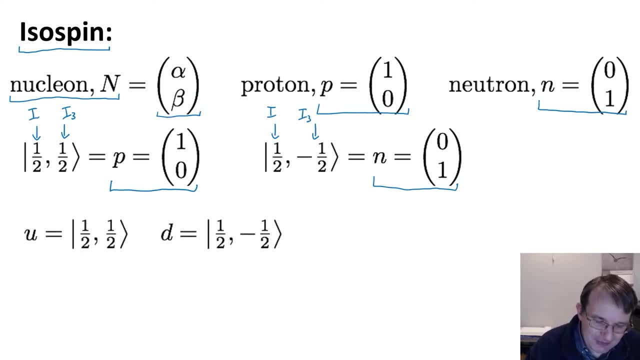 Now, fundamentally, we can take this symmetry down one step further and we can write the up quark as isospin a half And I3 plus a half and the down quark here as isospin a half and I3 as minus a half. 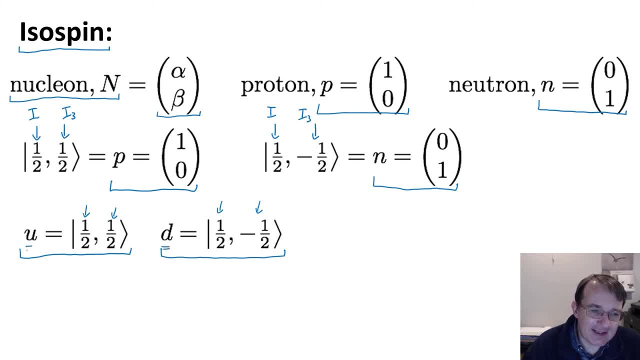 And again it's the same symmetry. The mass of the up and the down quark are almost identical, So we can think of this as some sort of light quark, light quark particle. And this light quark can exist as an up or a down state right, So it can either be in an up state in which 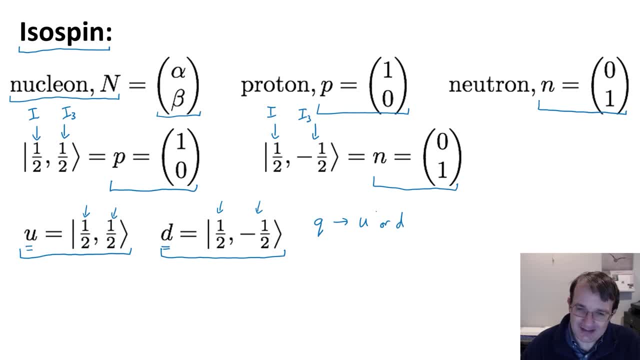 case it's got the, it behaves like the up quark, or it can be in a down state, in which case it's like a down quark. So it's an artificial construct, but the way we can get away with it or the reason we can, 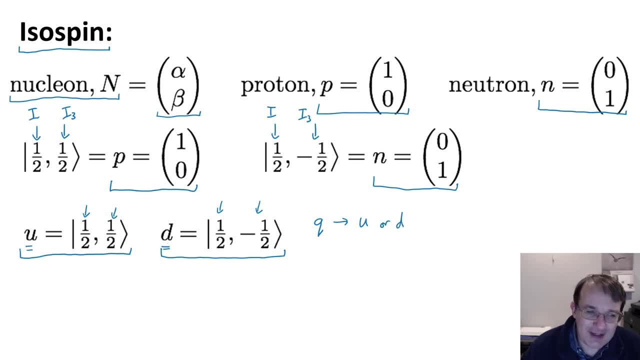 get away with. it is because of this accident where the up and the down quark, or the proton and the neutron, have almost identical masses. And the reason this is useful is because the strong force conserves isospin right. So if we have a strong force interaction, we conserve isospin. So the isospin before is equal to 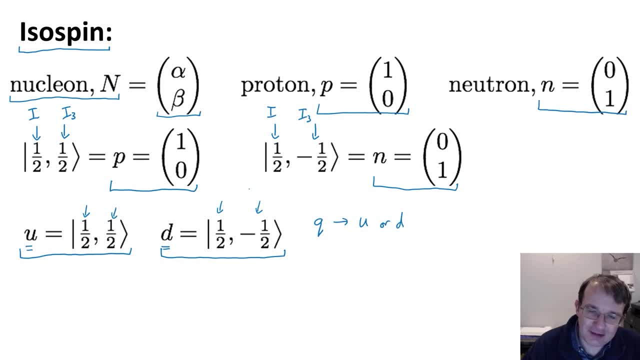 the isospin afterwards. It's also useful in determining whether states, whether certain bound states exist and whether certain interactions are allowed to occur, Because you can rule out certain interactions by looking at the isospin symmetry and discovering that, no, this interaction is not allowed because it under the strong interaction, because it violates. 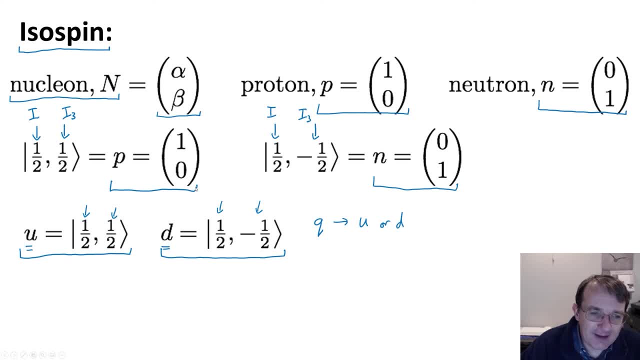 the isospin symmetry. Now, because the three component of isospin is associated with the number of protons and neutrons, or up and down quarks, we can actually use this three component to calculate the charge of a particle. So this is the total charge and it's equal to the third component. 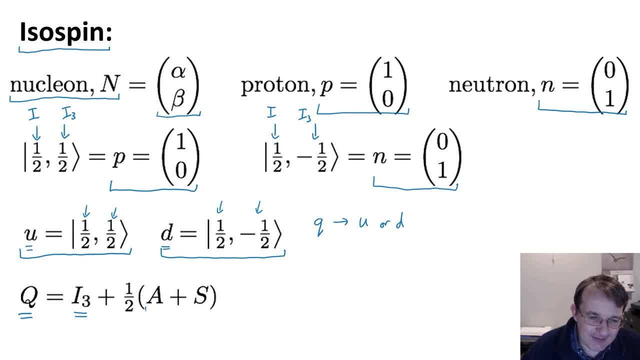 of the isospin of the particle And then plus a half. this is the baryon number Right. So this is the baryon number and this is the strangeness. And we have to include the strangeness here when we're calculating the charge, because the strange quark is not. 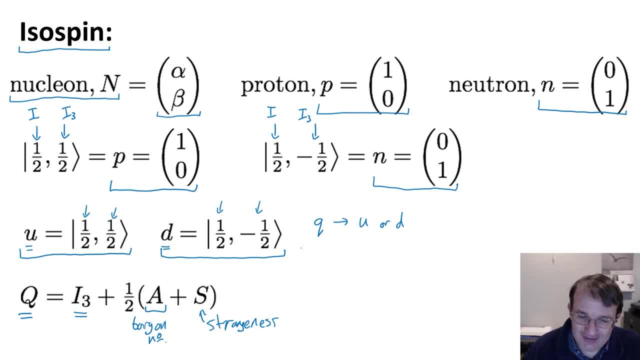 part of the isospin symmetry right. So it doesn't have an isospin at all, but it does have an electrical charge. So we do need to include the strangeness here And we also need to add in the baryon number to get, because this essentially accounts for the number of 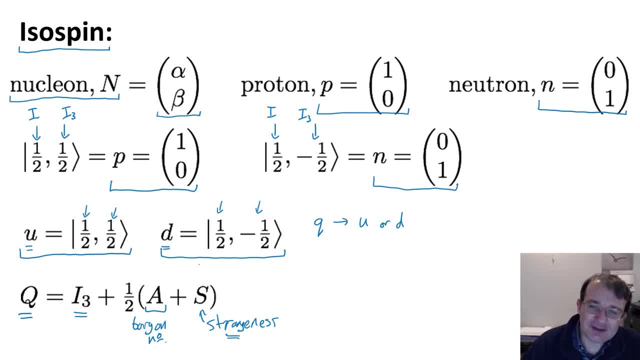 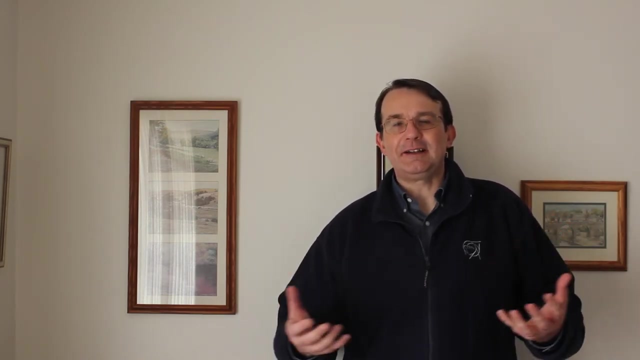 quarks that we have. So isospin is a very useful symmetry when dealing with up, and predominantly up-down, and some strange quark states operating through or decaying or being created through strong interactions. Now, as we mentioned, the reason isospin is so useful is because under strong interactions, 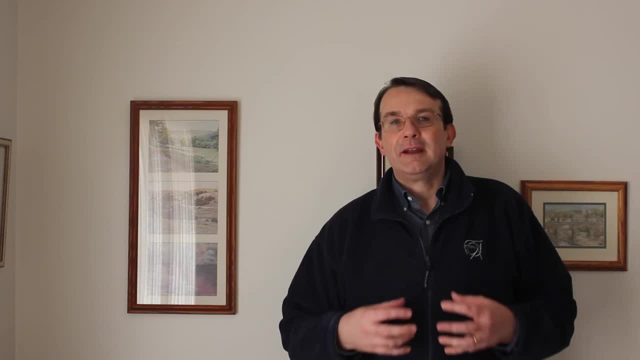 isospin is not. Isospin is conserved. Now, if we wanted to extend isospin and say, well, what about the strange quark? It's not that much more massive than the up and the down, then we could start to imagine some. 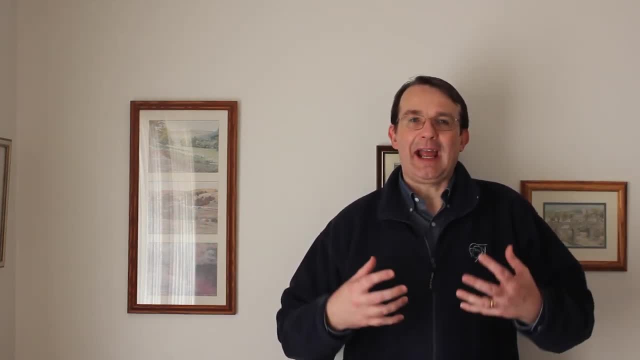 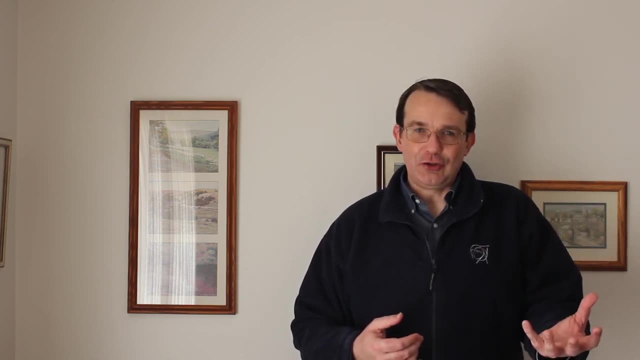 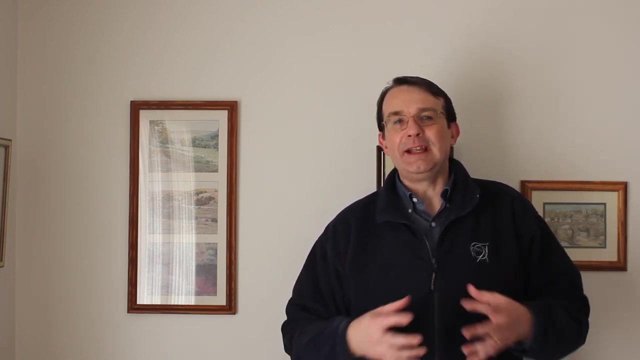 sort of extended isospin which would have a quark that could be in one of three states- up-down or strange- And when we have two states, an up and a down, then the symmetry we get is called SU2.. When we extend it to three, then you get a symmetry called SU3.. 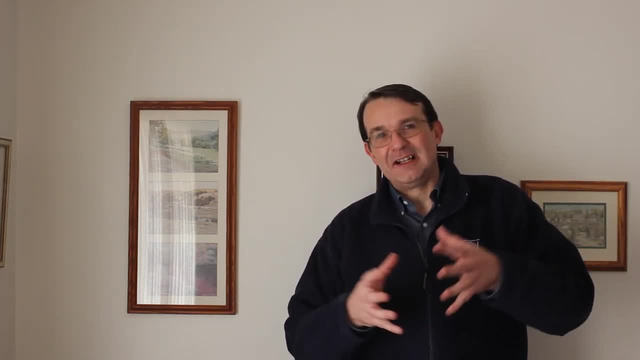 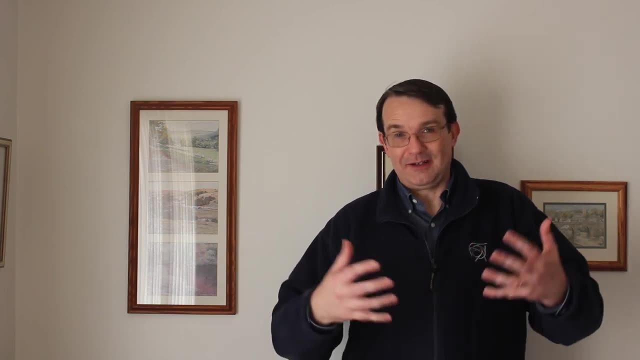 The problem with that is that, while the strange quark is just a bit more massive than the up and the down quarks, it is noticeably more massive It is. you know, it's actually quite a noticeable difference and that has an impact on the masses of particles. For example, a lambda zero baryon which consists of an up, a down and a strange is quite a bit more massive than a proton or a quark. So that's the problem. It's not the same as the up and the down quarks. 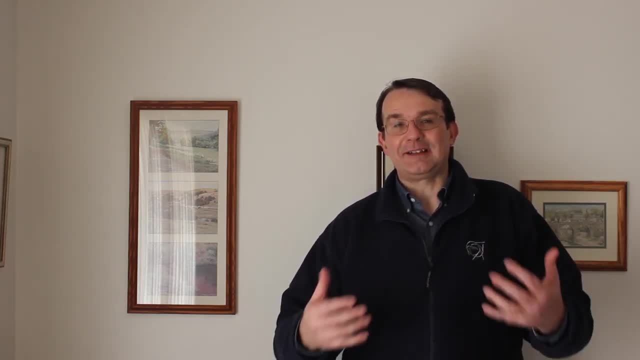 It's just that the symmetry is much more massive than the up quarks. So you know, the problem with that is that the symmetry is much more massive than a proton or a neutron, And it gets worse as you extend it further. If you try to extend it to SU4 and include the charm quark, the symmetry hits really. bad. and it's even more broken if you extend it to SU5 and include the bottom quark. and it is utterly broken if you try to go to SU6 and include the top quark, because the top quark never actually forms any bound states whatsoever. 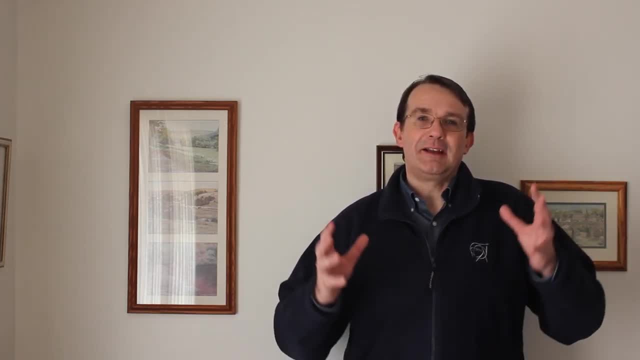 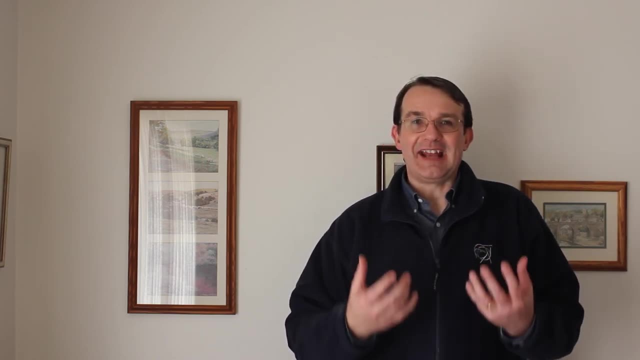 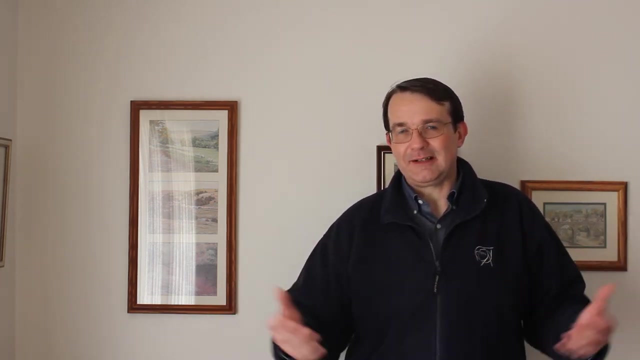 So that is completely useless. So, generally speaking, you will never see. You know, isospin is just restricted to the two light quarks, the up and the down, and it's an SU2 flavor symmetry And we don't include any of the other quarks because the symmetry basically doesn't work. 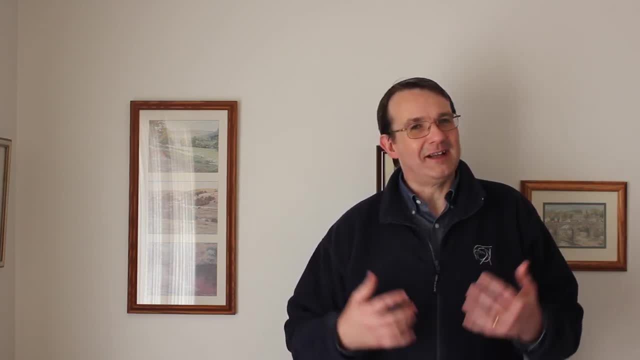 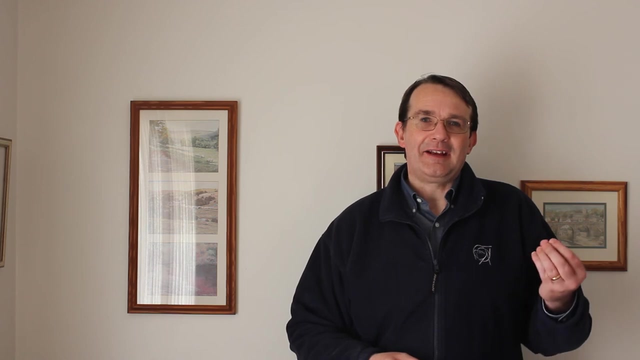 if you do, because these quarks have different masses and we can't treat them as different states of the same particle. So that's it for our first symmetry on the Standard Model. However, the Standard Model is built on relativity, And relativity itself actually has symmetries. 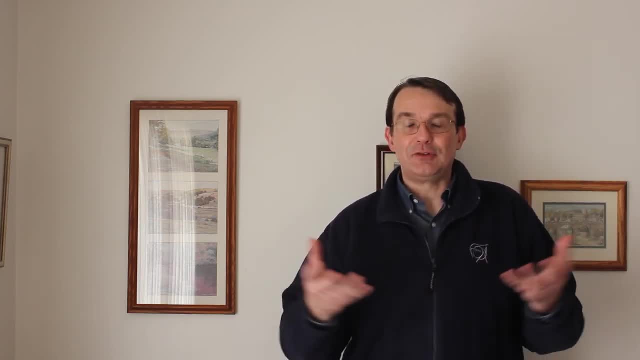 The Lorentz boost vectors, the 4x4 vectors that boost between frames. they form a Lorentz group and there is a Lorentz symmetry associated with that group And in the Standard Model, those fundamental symmetries we refer to as CPT symmetry. 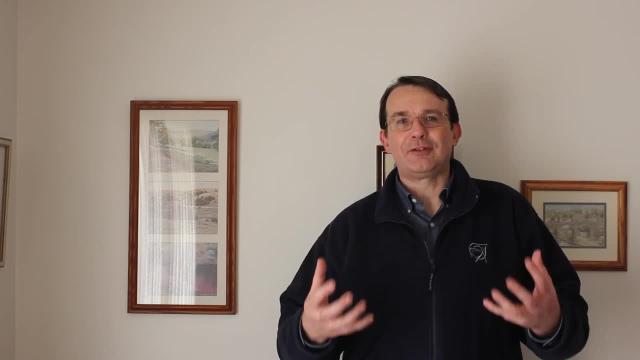 And in the next video we'll start to discuss how those fundamental symmetries were studied and what we found out about them.